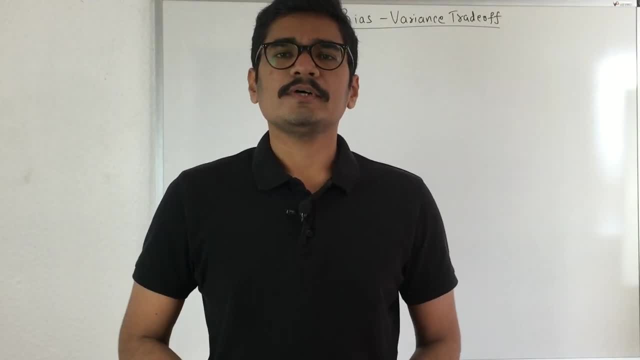 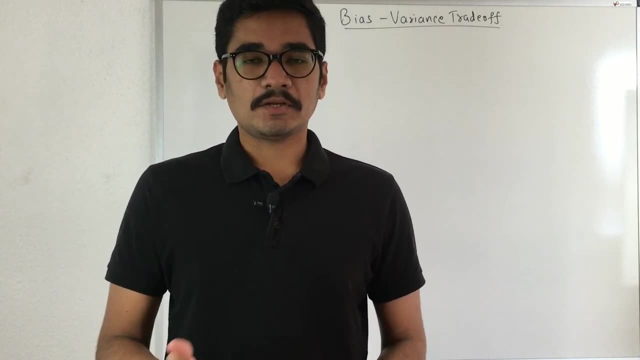 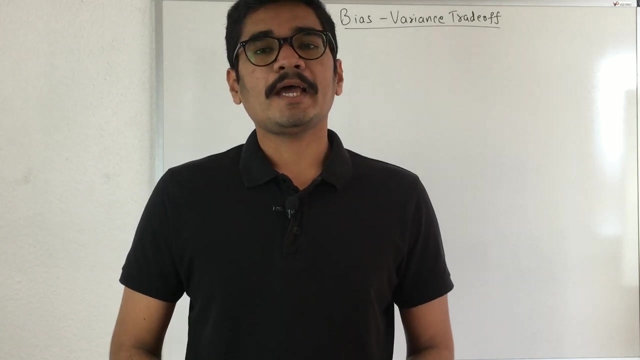 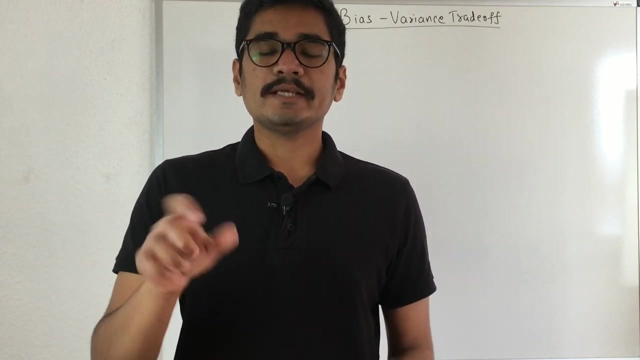 Hello people, welcome back to my channel. So we have done so many things in machine learning so far. We have seen different types of machine learning models, including linear regression, logistic regression, and also we saw some of the videos of decision trees, how it is implemented, and we saw some of the conceptual things in this. So, while we develop these models, there exists a concept which is called as the bias variance tradeoff. So that's not. 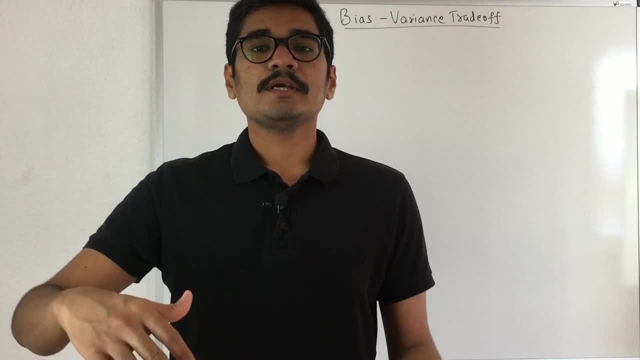 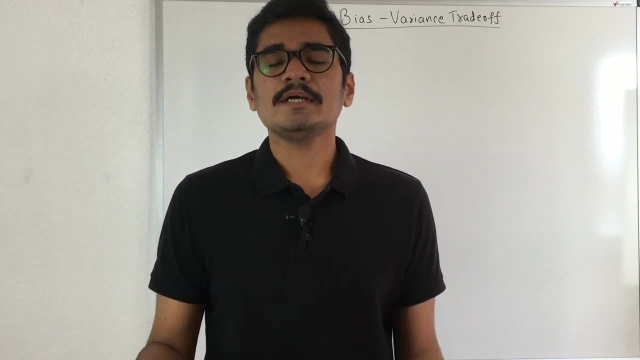 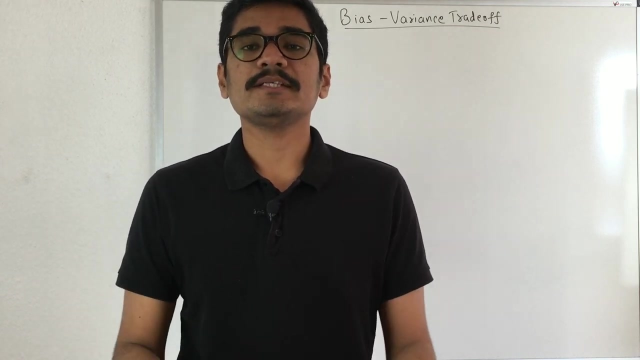 with the machine learning models that we build, but in the nature itself, whenever you buy something or whenever you are doing something, some are here. you will get to know that these things already happened to us but we never knew like. this is called as the bias variance tradeoff, but only when we learn into machine learning or when we see these terms- that is, bias and variance in machine learning, we come to know, okay, this is called as the bias and variance. So 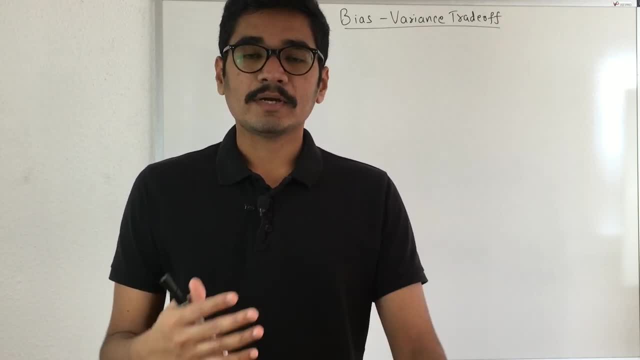 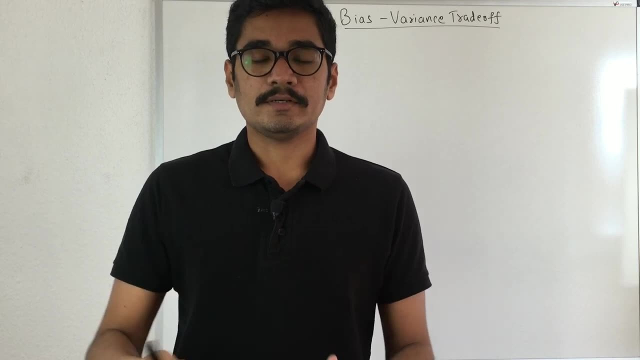 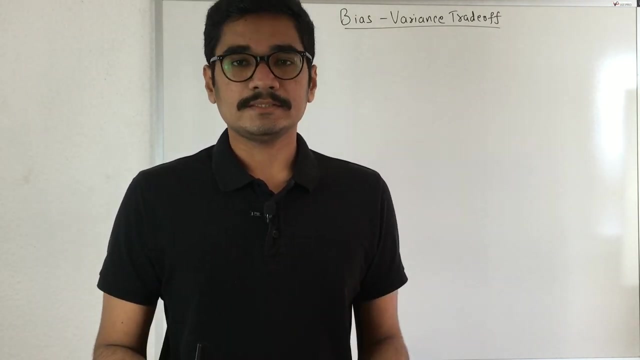 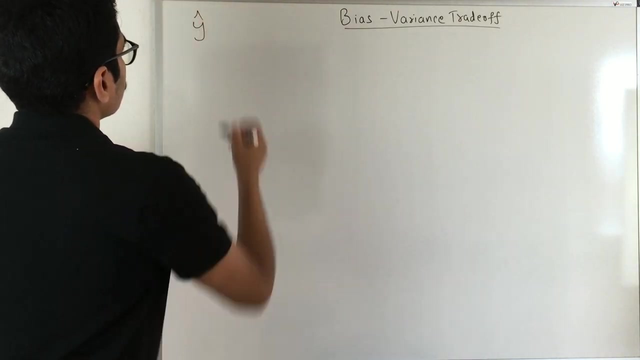 today in this video, my focus will be to make you understand the concept of bias and variance tradeoff, and you can then understand how these are important while building your machine learning models. Okay, So for bias and variance tradeoff, we'll take a simple example of linear regression model. So we want to predict something? Okay, So that is my Y cap and I have coefficient, say, beta naught plus. 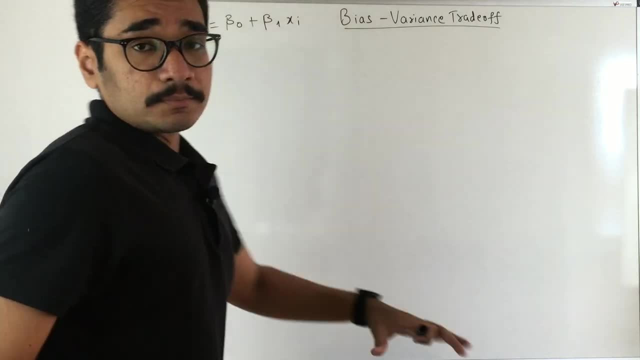 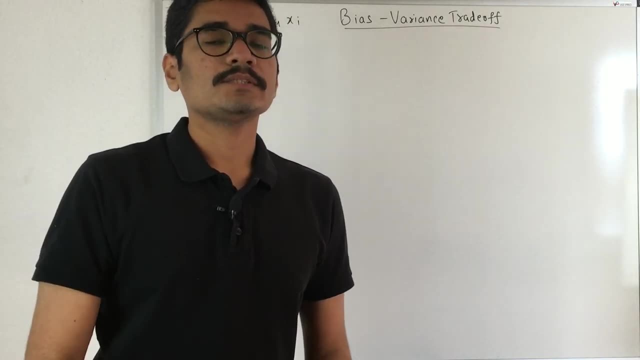 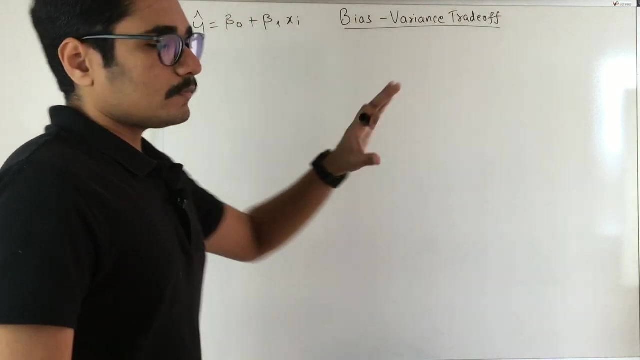 1, X, 1 or X I. so this is my general formula for estimating or for predicting anything. So you can do forecasting as well, but here we are not doing a forecasting, but we are doing a simple prediction. So now, what are use cases? say, I want to purchase a new laptop. 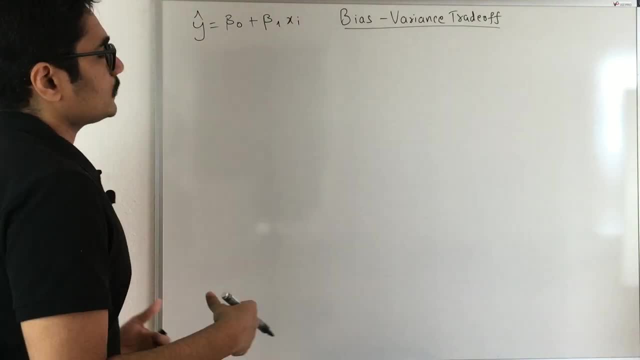 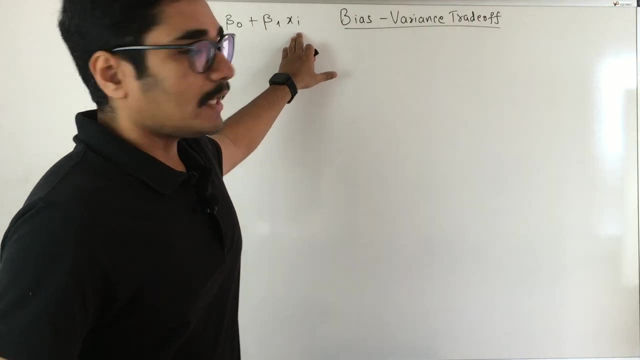 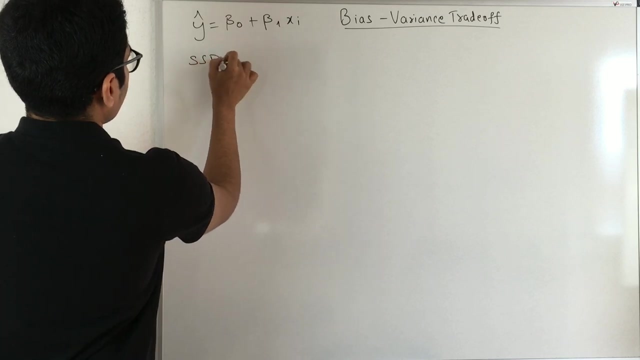 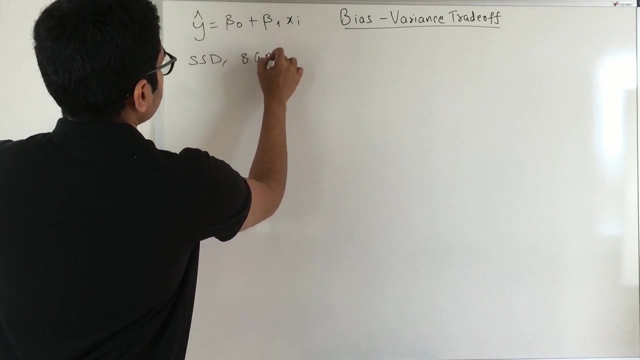 So while purchasing the new laptop, I will have saved my own requirements. So those requirements are considered as my variables, that is my features. So say, for example, I want a requirement like it has to be a SSD, that is, solid-state drive, or it has to be with some RAM, that is say 8 GB and 3.7 gigahertz processor. 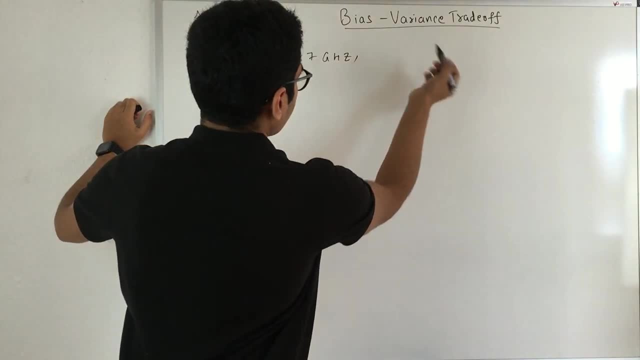 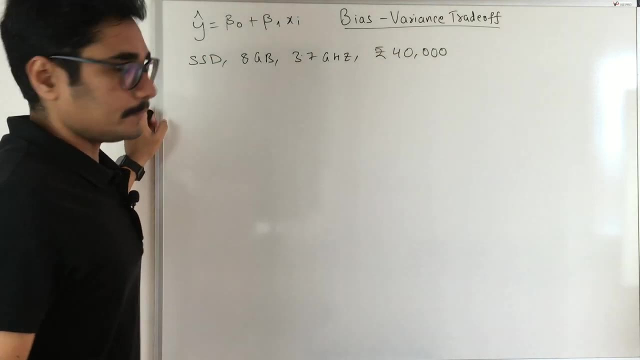 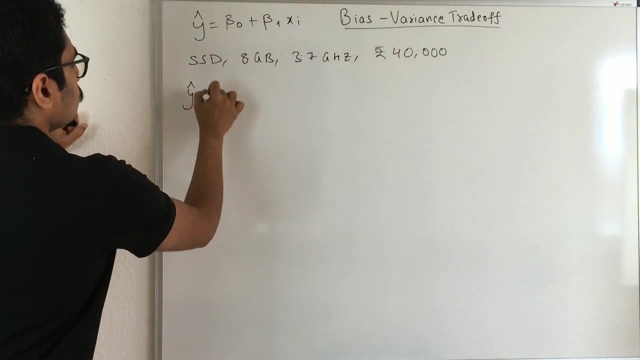 And finally, you want to have the price, say it is of some price. Say you have some 40,000 rupees approximately in this range. So if I want to make a model out of this, so actually you don't need a model, but just if 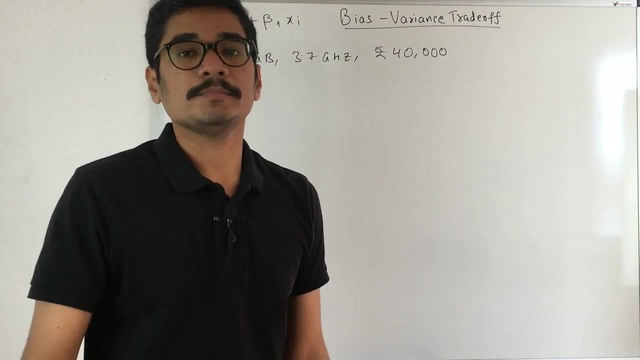 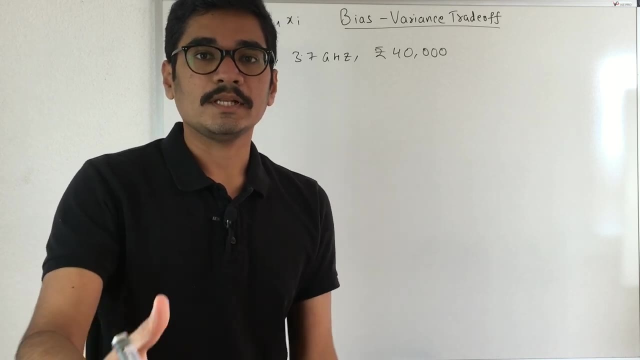 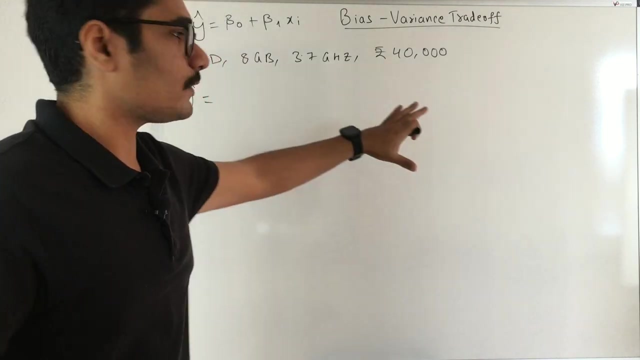 you have different varieties or different configurations of machine given but you at the end is having difficulty to predict like which model or which laptop to buy, then you can have this particular data set and you can basically build a model for your own activity. Just for that, okay. 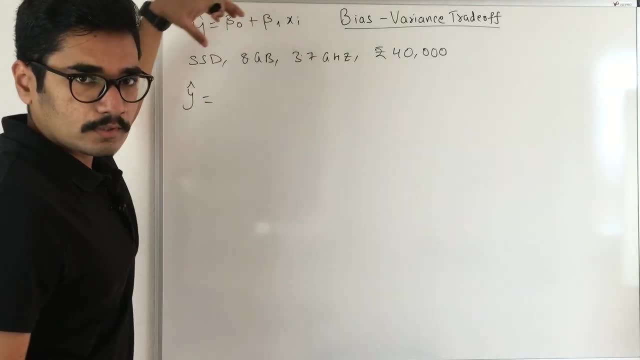 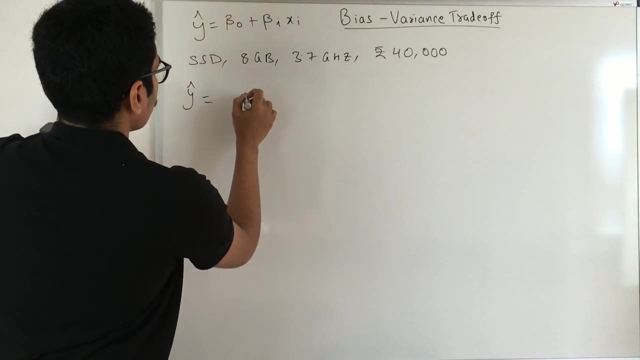 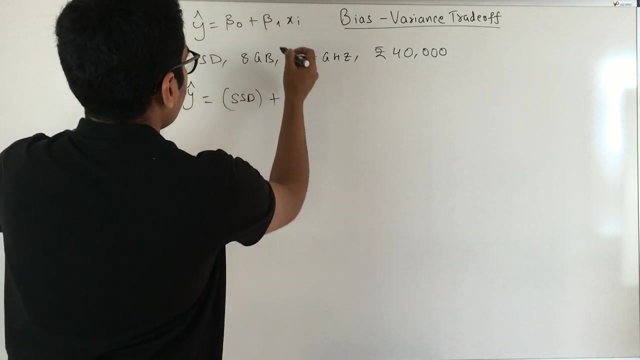 So say here: if I want to plug in this values or these are my features, and if I want to plug in into this equation for prediction, say, I have SSD, so for SSD I am writing it as SSD. Okay, so that is beta, not okay. and then 8 GB. 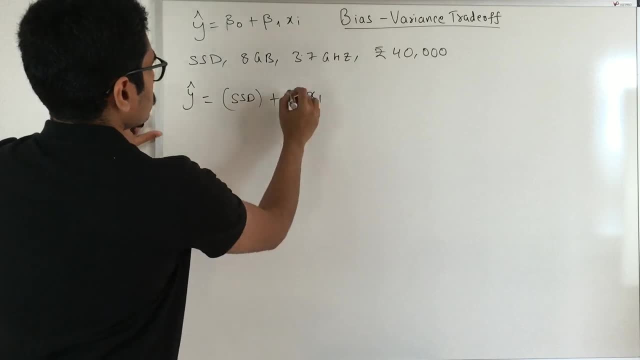 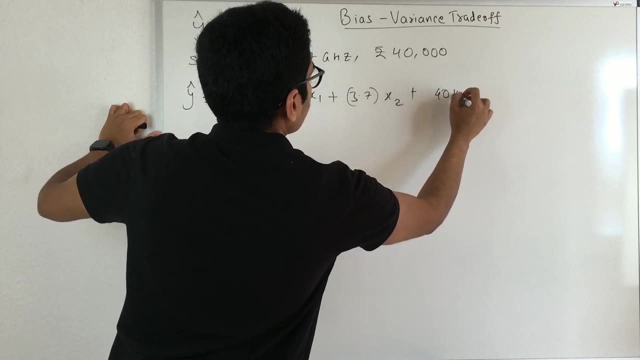 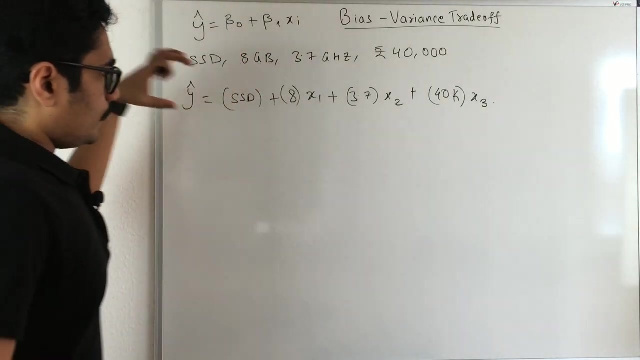 So with 8 GB, I have saved x1.. So I'll write in this way: and 3.7, that is x2.. Okay, And this is 40,000.. This is x3.. And with this, what happens is like when you see this particular thing, or when you are. 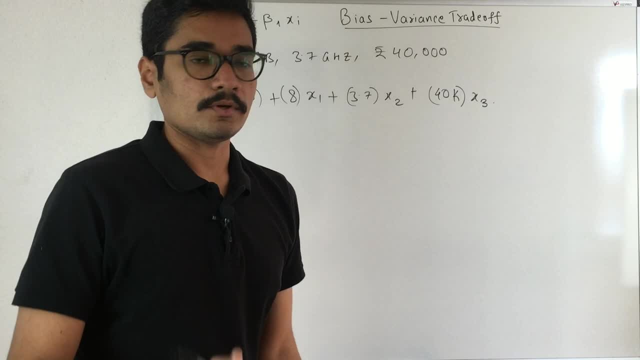 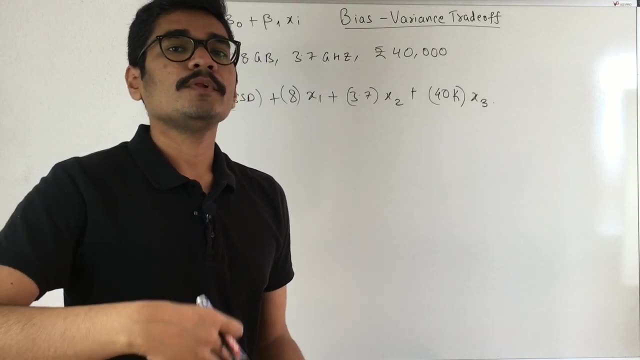 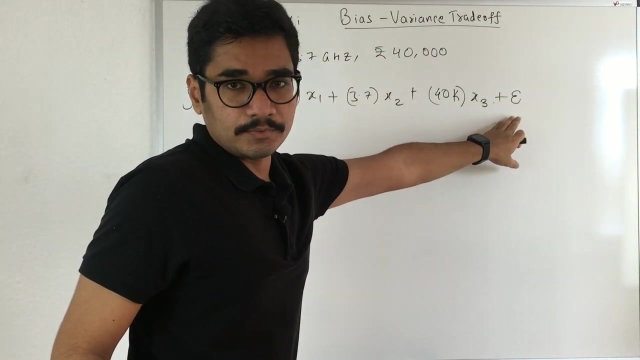 satisfied with these many features of one particular laptop that you are getting here or there. there would be some errors, or when you buy something, it will not always be satisfactory. So for that we are incorporating some errors. Say, for that We are using Epsilon. 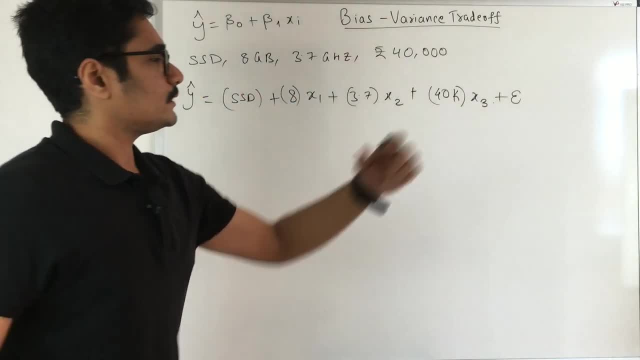 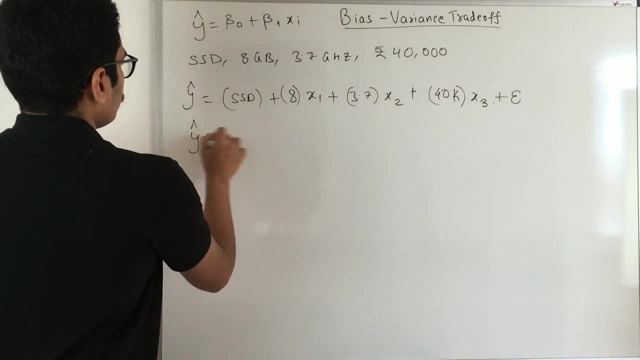 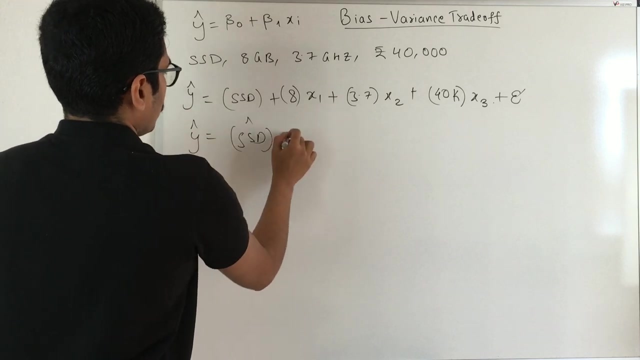 So now we say like, okay, I just don't want the error, I'm not concerned with the error, I just want these many features. So what I do is I will have an estimate of all these things. So I will now eliminate the error in the next step and say I have SSD cab plus this cab. 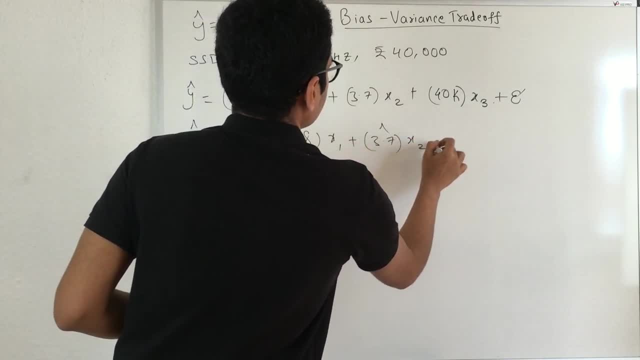 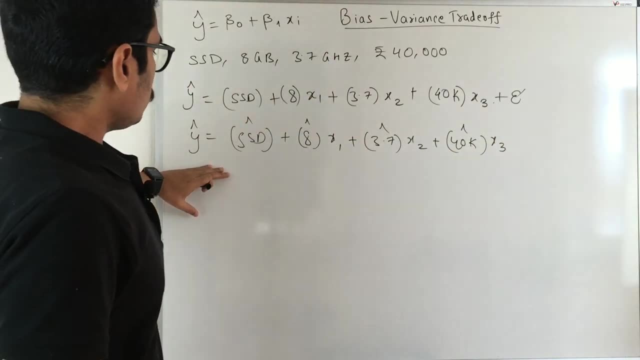 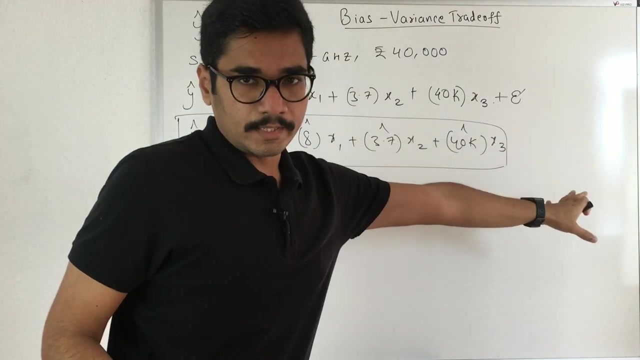 something, something. okay, So this is the estimated one that I'm now writing, So my error In this case won't be there. Okay, So now this is my new prediction for buying a new laptop. ignoring the error or this cab means like you have estimated the error and you are incorporating. 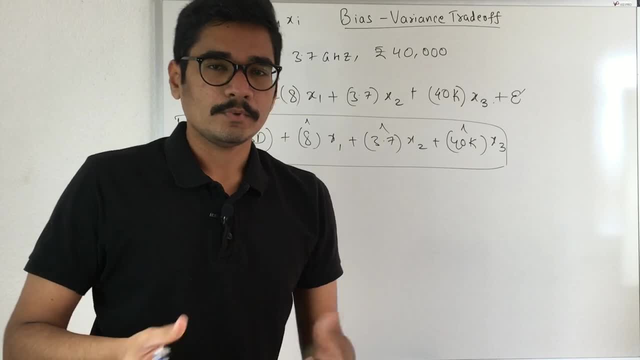 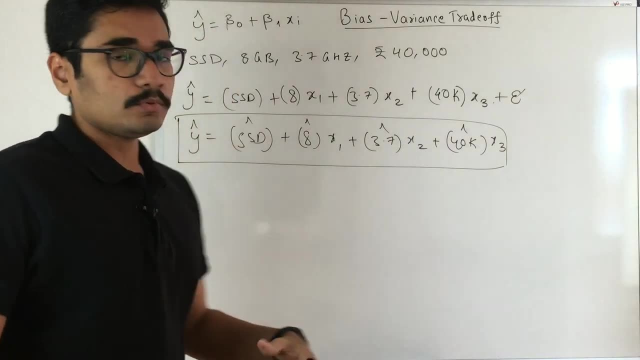 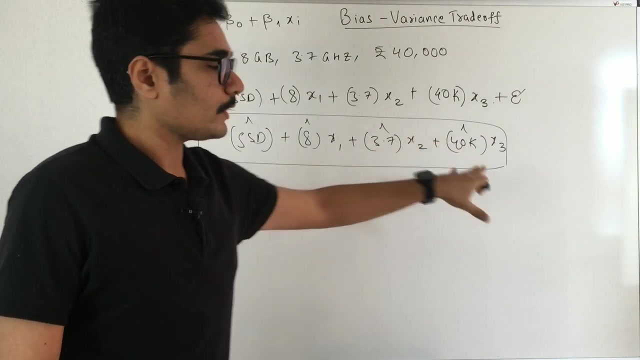 Okay, It's here on there, like something above or something below. I'm okay with that. Okay, Now you know like, in order to predict, or if you want to make your model predict, you need Many parameters. that is, this beta naught, beta 1, beta 2 and beta 3. now my question is: do? 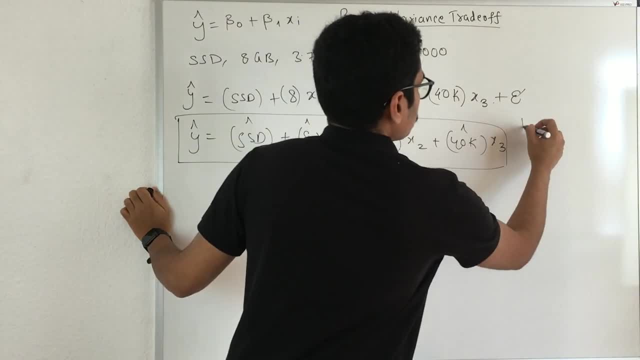 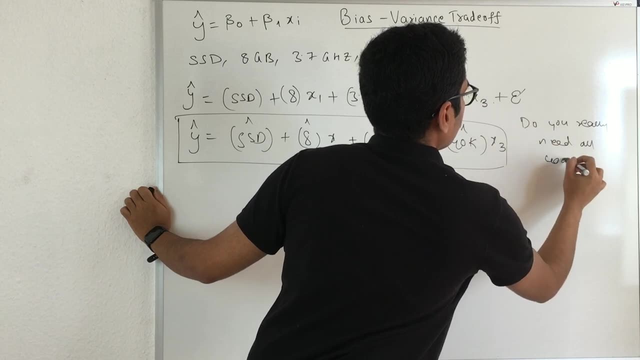 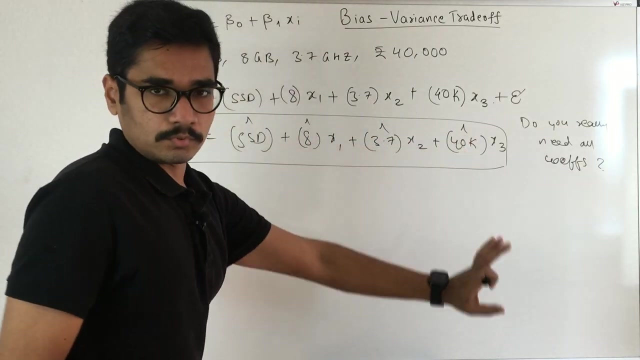 you really need all this coefficients? So do you really need all coefficients? So this is my question. So now here, since you have 1, 2, 3 and 4 coefficients, do you really need 4 coefficients for their model to predict? 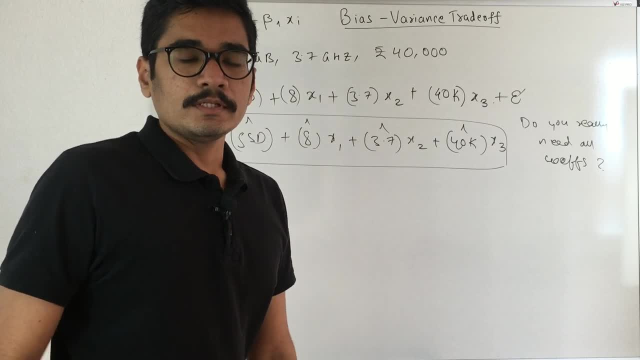 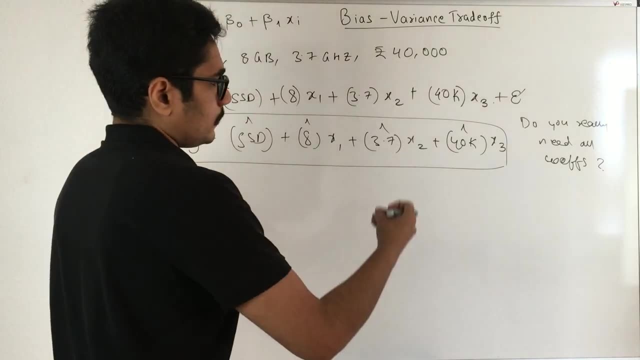 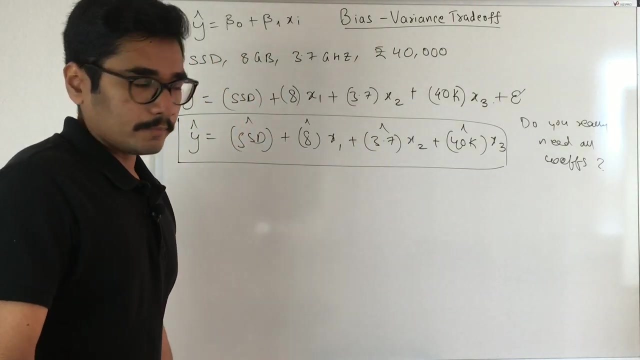 In some case, if you make all the coefficients as strict, then it will say, like I want all the coefficients, then only I can make the prediction. but what if I say, if I give only two predictor variables or if I give only two features, whether it will predict or not? 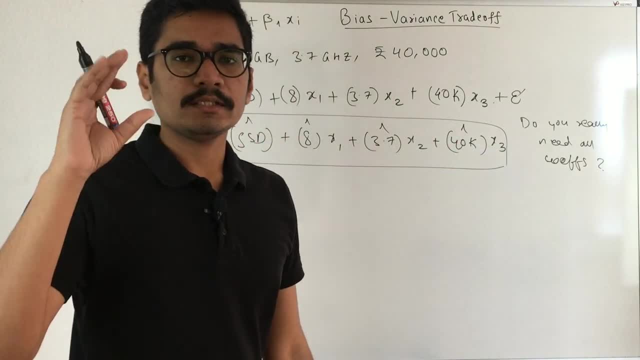 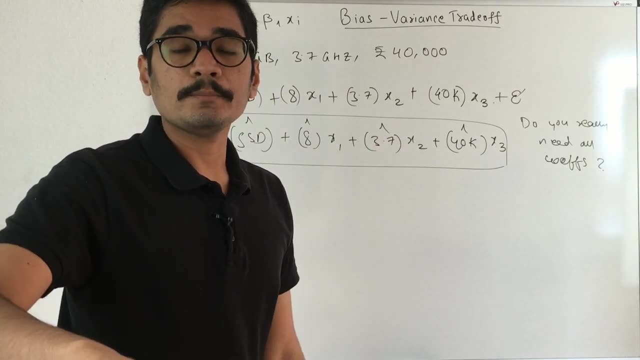 Okay, So ideally, if you give all these parameters, then the ideal case that should happen is it should predict correctly. but if two or three parameters are not given, or if you are making use of only two or three Predictor variables out of this, then there could be a chance like your prediction is. 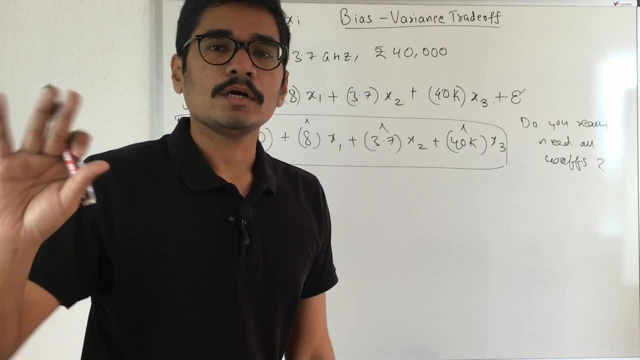 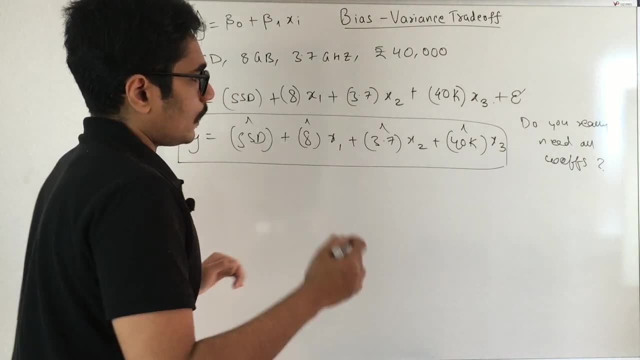 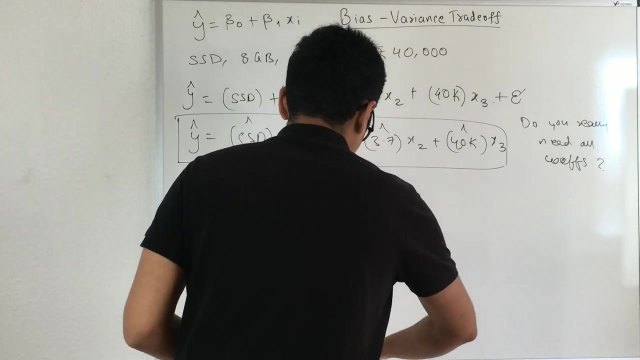 wrong or it would predict you some different configuration of different laptop. So that is one case that is happening. Okay, So now, how significant for you to drop that input feature or predictor variable, So say, for example, if I drop this price, I'm not concerned about this price. 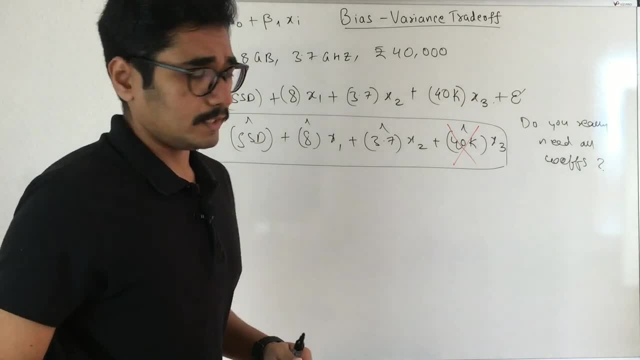 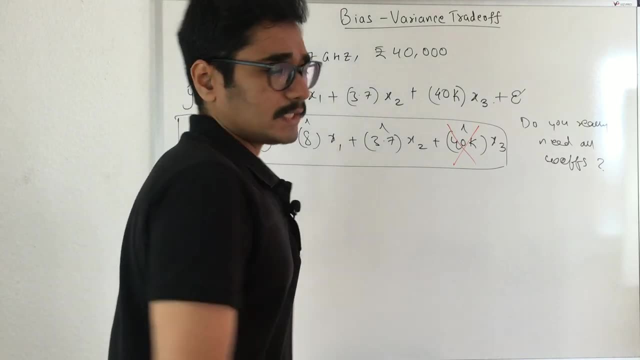 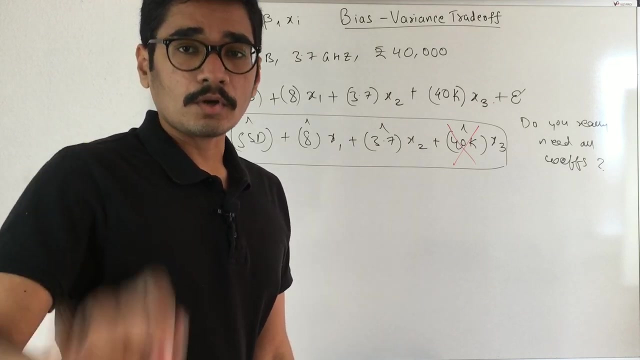 So I want SSD, I want 8 GB RAM, I want 3.7 gigahertz. I'm to the least concerned- or I'm least concerned- with the price range, So I'm not concerned about the price. So dropping a particular input feature requires justification why you need to drop that. 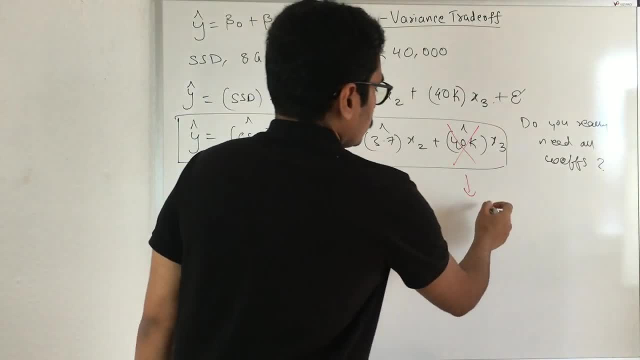 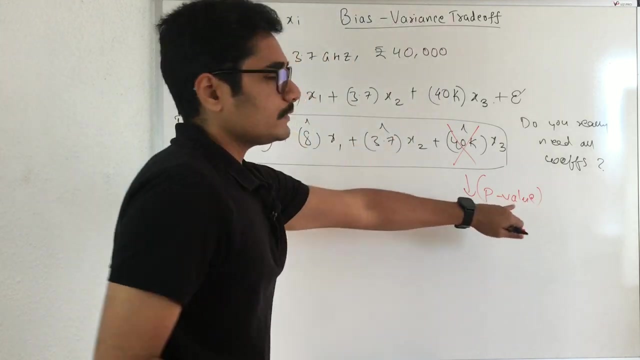 So if you need to drop this, so say, for example, you have to test its significance, So that is called as significance testing in statistical literature. So there you have. You have some coefficients, say you have a p-value, So here p-value is not associated in this scenario, but p-value is mostly used in medical. 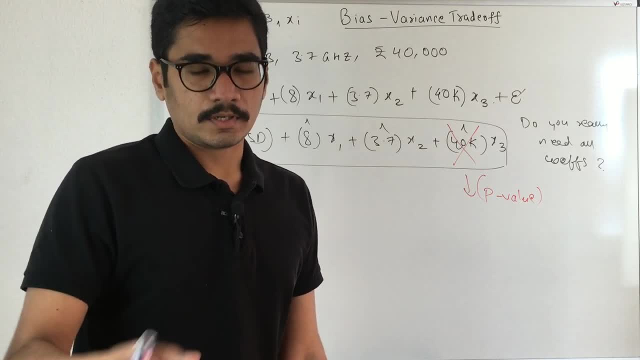 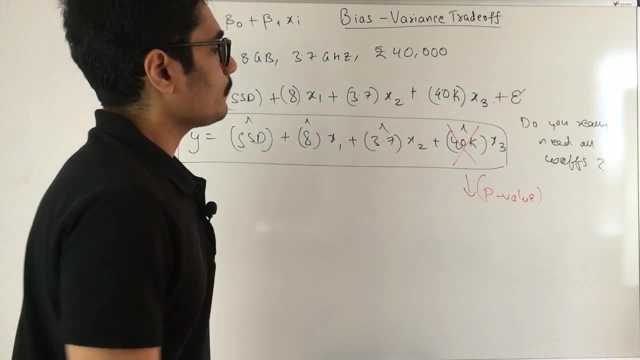 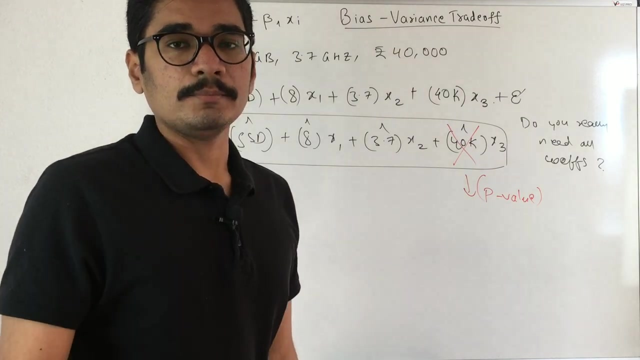 cases where you want to test a drug or like you want to produce a drug for some treatment. So their p-value indicates like it is most significant. So say, just in this case, for your understanding, we take the p-value for checking how that predictor variable is going to be significant. 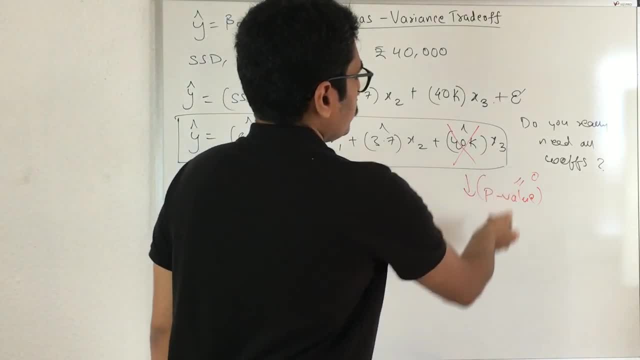 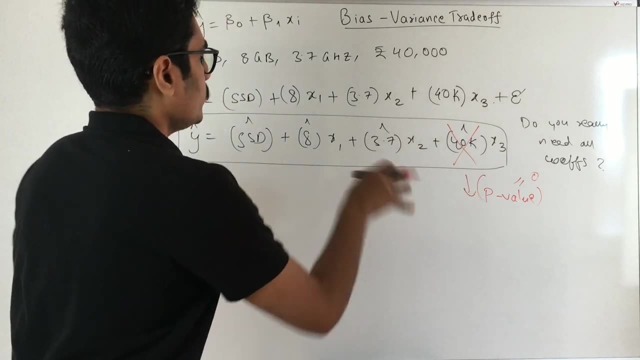 Now, if p-value turns out to be 0, so that means that predictor variable is no more required for your prediction and you can basically drop off. So in that case, if you want to make any prediction, you are good to go with these three parameters. 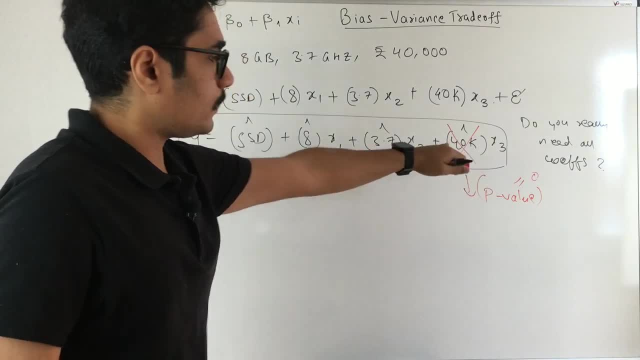 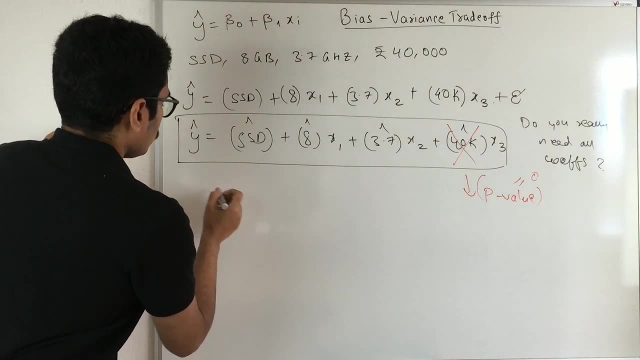 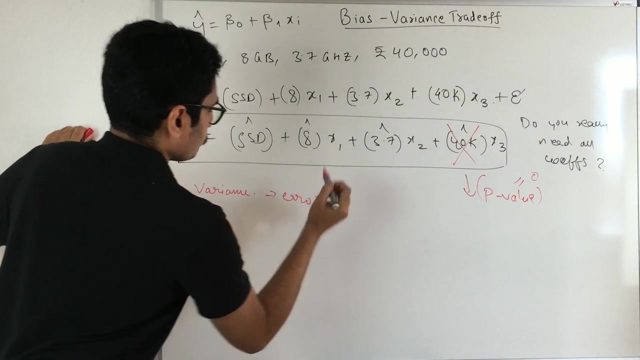 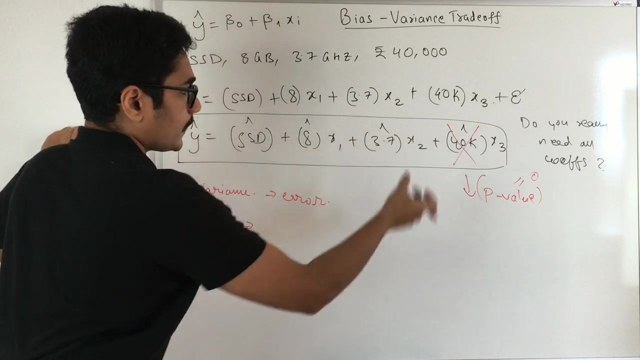 You need not have this final price column or the price features. So what happens is like you want to have a variance, So variance will be there. So that is nothing but your error. Okay, and you have bias. So bias means like you initially thought, like you will predict with all this for parameters. 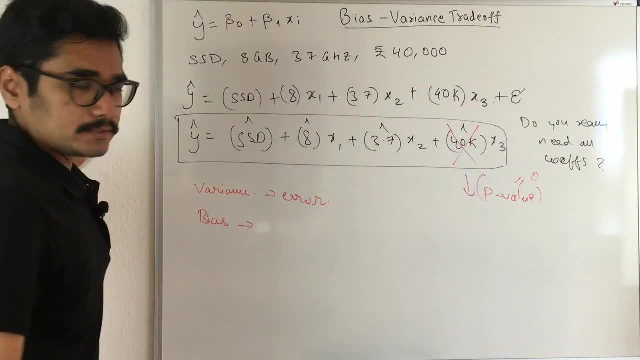 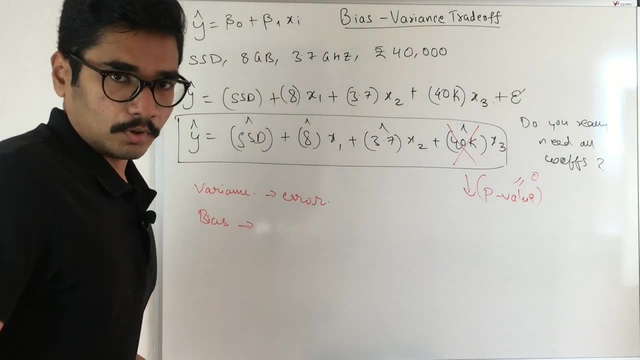 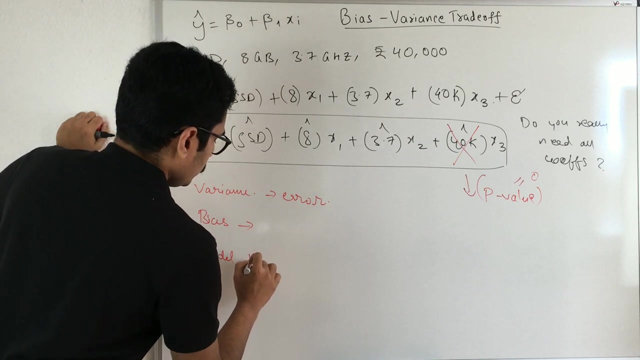 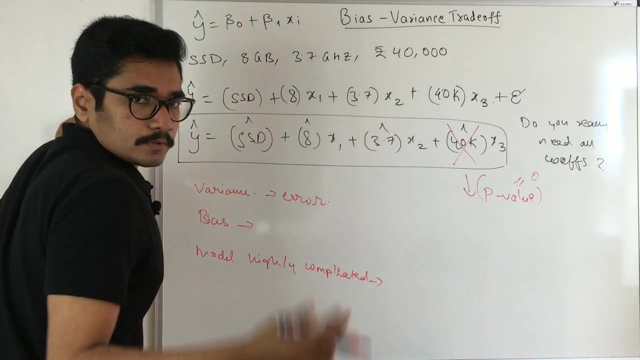 but you are, at the end, compromising on one parameter, So that is nothing but your bias. Okay, So for this, how will you basically model this? So now, if you have a model Which is very highly complicated, okay, so if you have built a model that is very complicated, 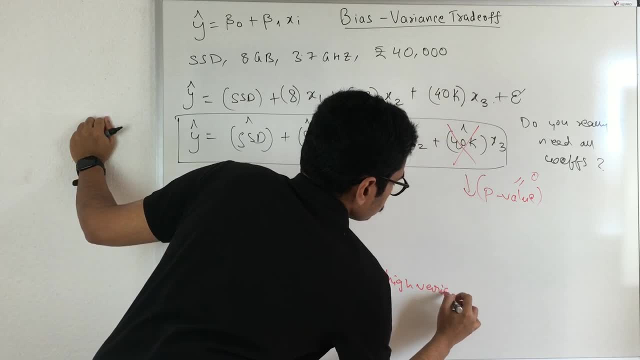 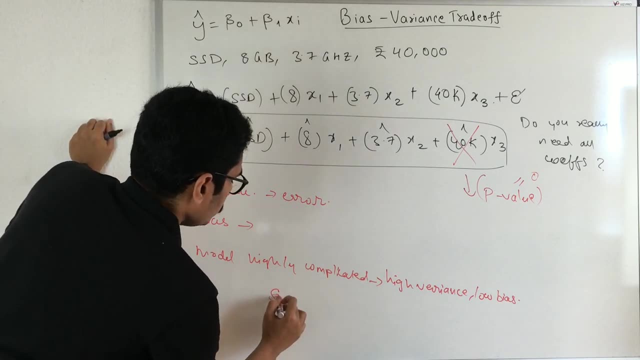 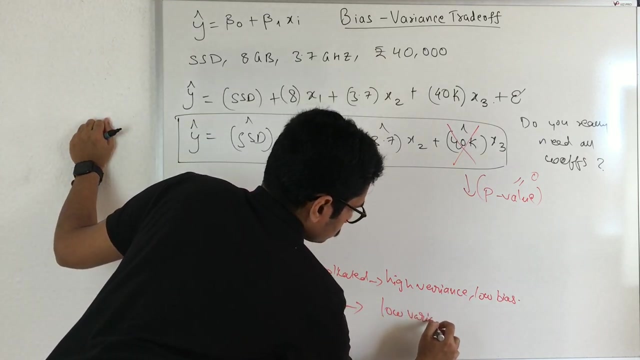 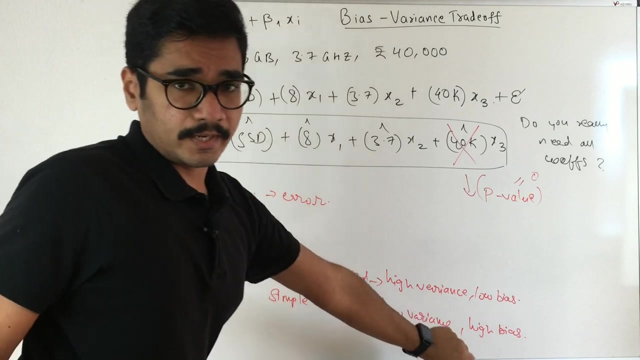 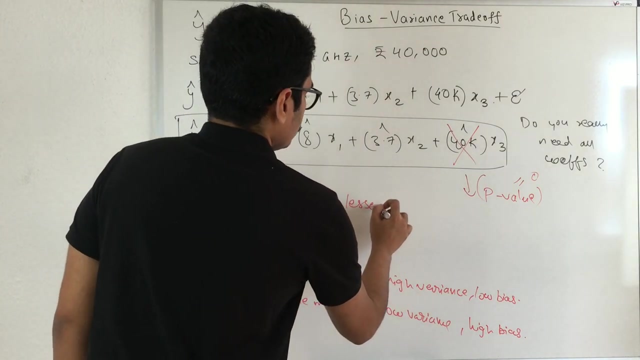 it will have high variance and low bias and, on the contrary, if you build a simple model, then Then you will have low variance and high bias. So this is the fact actually. so now our major goal is to have lesser variance. So how will I have lesser variance? 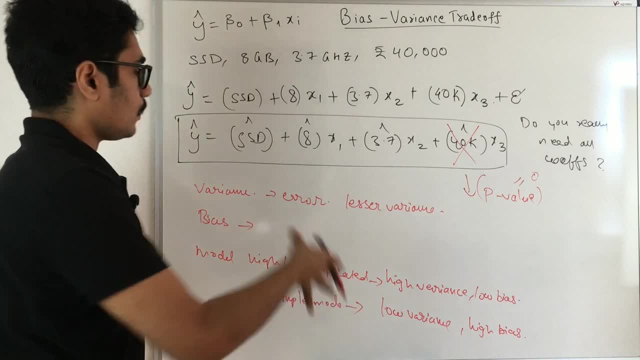 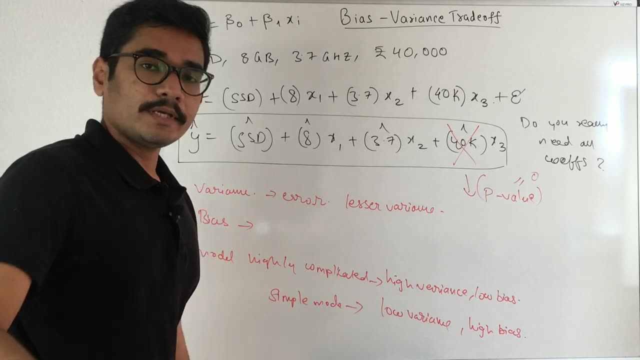 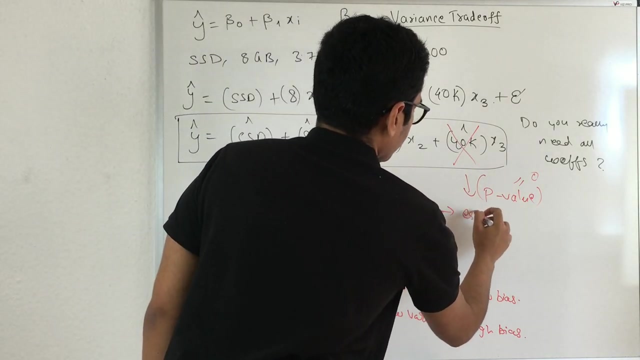 So in this case, if we predict some model or if we get some configuration of a laptop, and if we have variance, but we want to reduce it, So how we can reduce it? by dropping off any of the predictor variables from the equation. So lesser variance means you estimate. 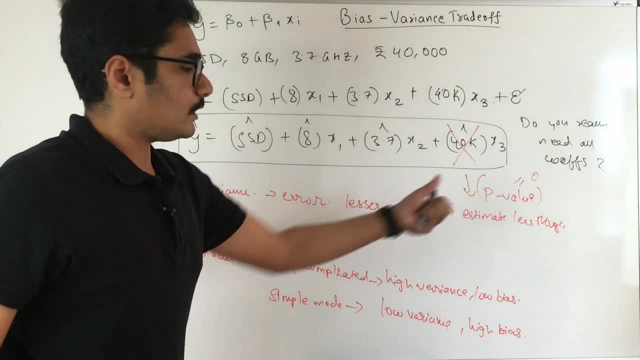 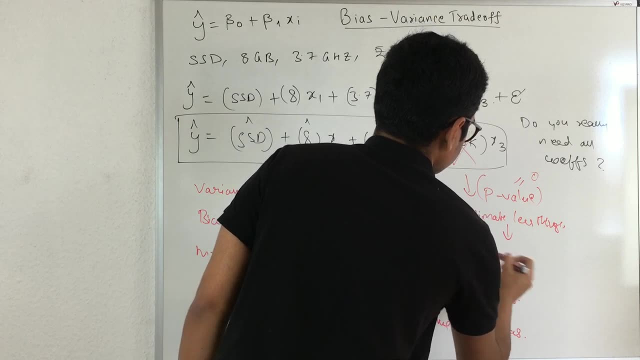 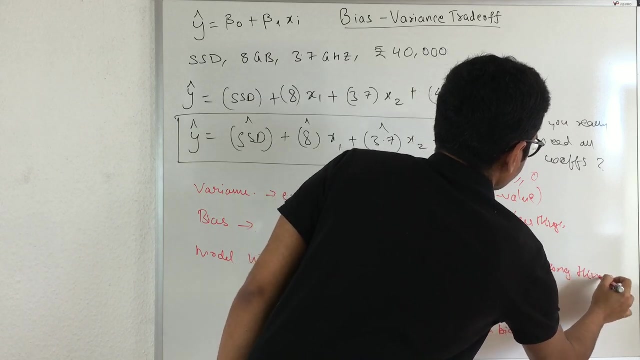 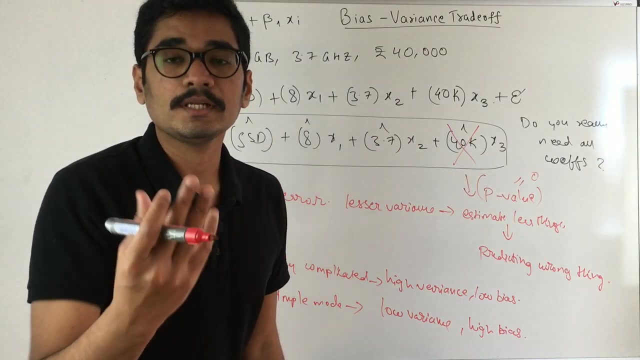 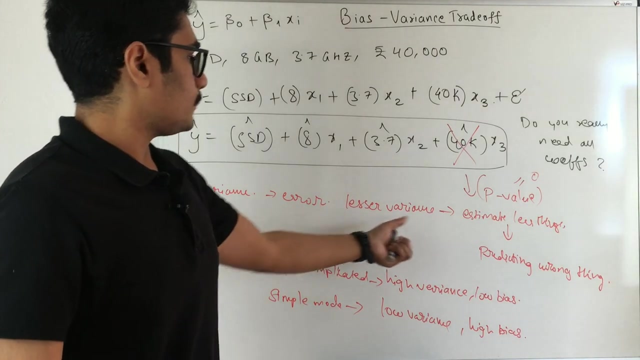 Less things or less coefficients or less features. but as soon as you estimate less things, You are predicting wrong thing, Okay Okay. So by giving all four features, your model could predict the right configuration or the right laptop, But since you are dropping one, you are predicting something wrong, because you are very much 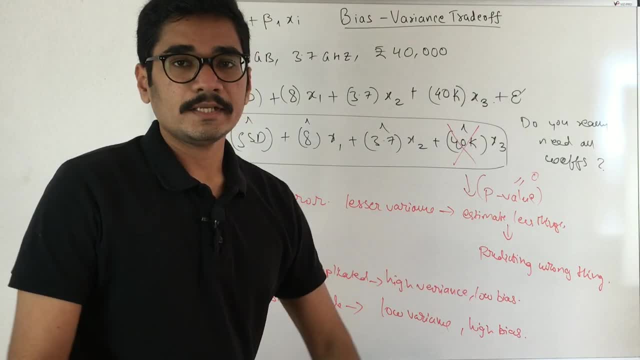 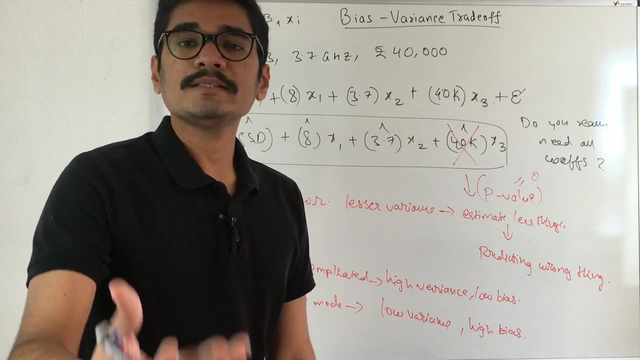 concerned about the variance, but your model is saying: if you are not giving all the four coefficients or all the four features, how can I predict you a good laptop or how can you suggest a good laptop? So in that case You are introducing some bias also. 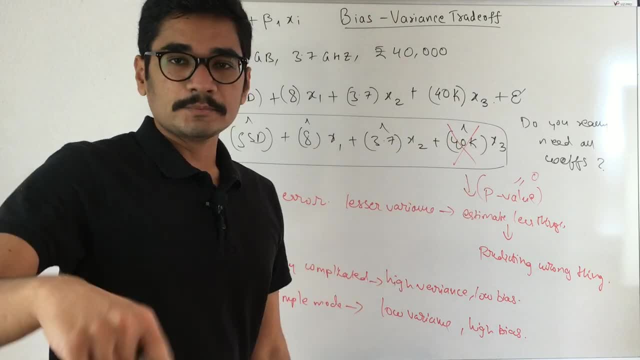 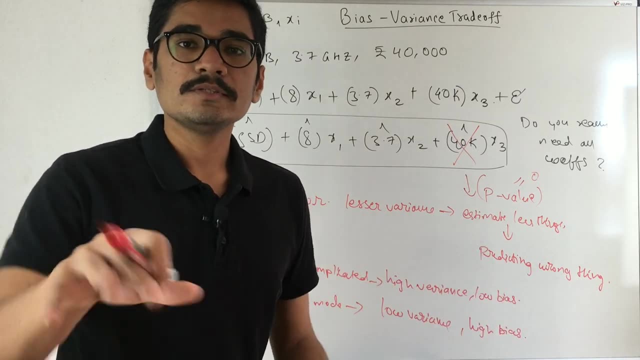 So you are not providing all the four coefficients, but you are just providing three coefficients, and you want smaller variance, but you are not concerned with money also. So these things in the real life also happens sometimes some days with you. So this is nothing but the bias variance trade-off. 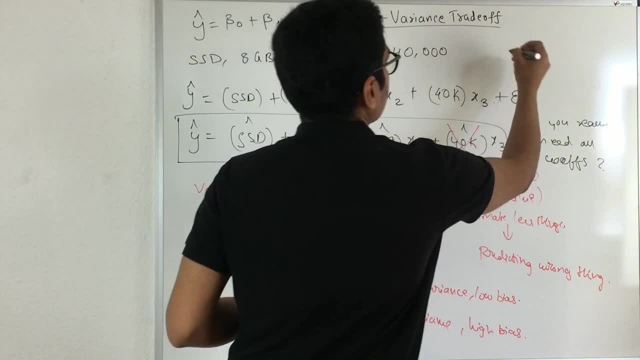 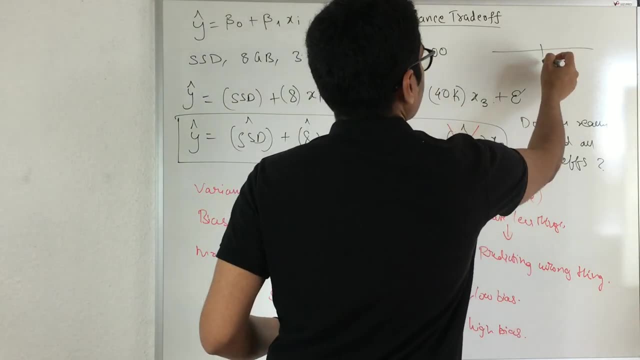 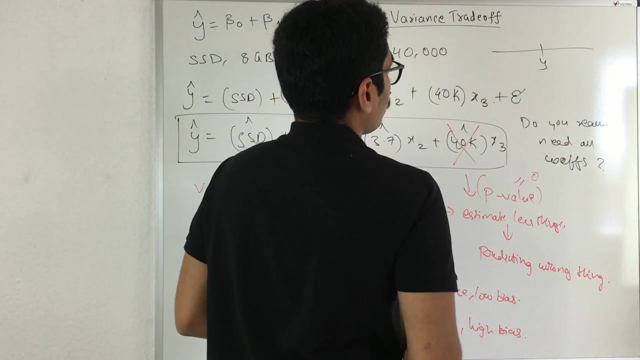 So if I give you something like say you want price estimate of some laptops, say you have a particular budget And say this is my wife, Okay. and if I ask you which is a better estimate of this, and if I give you a range, whether 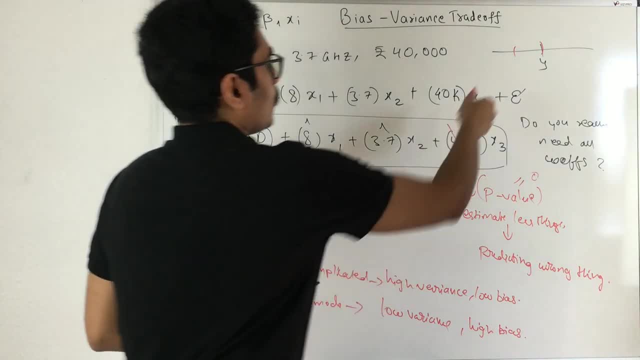 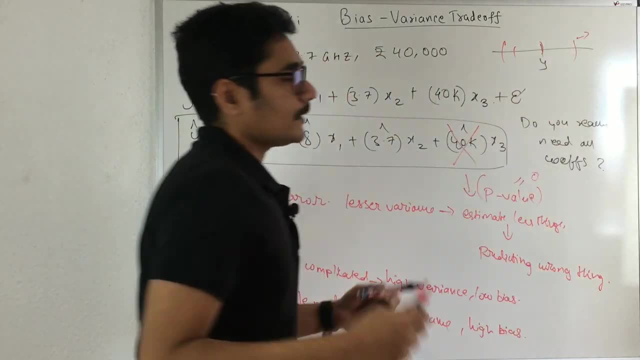 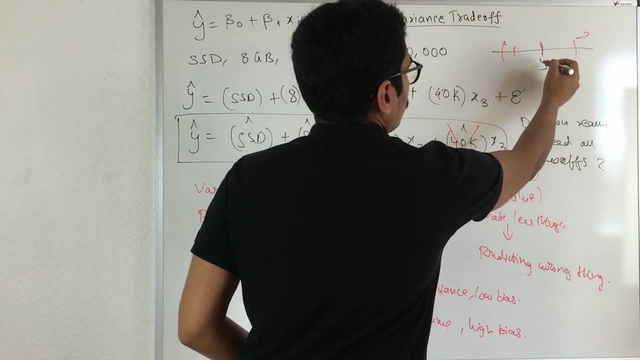 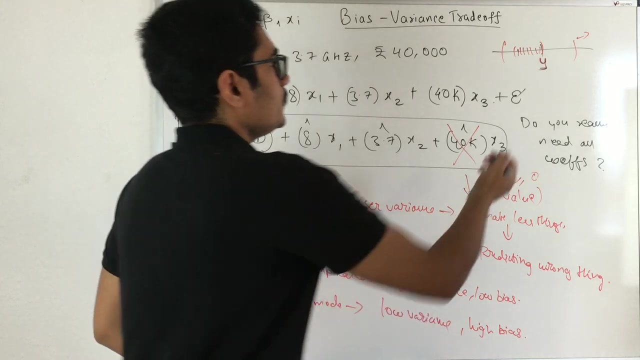 it is this estimate, a better estimate, or this estimate? So obviously the correct answer is the second one, because it will give you a wide range of different values in between. So if your actual budget is this, Okay, This much why. and if you are looking for price arranges in between this, then probably is. 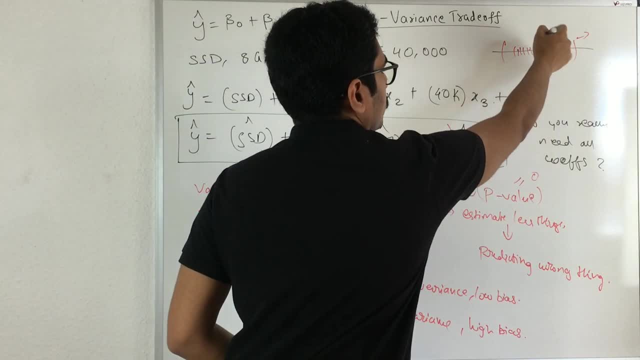 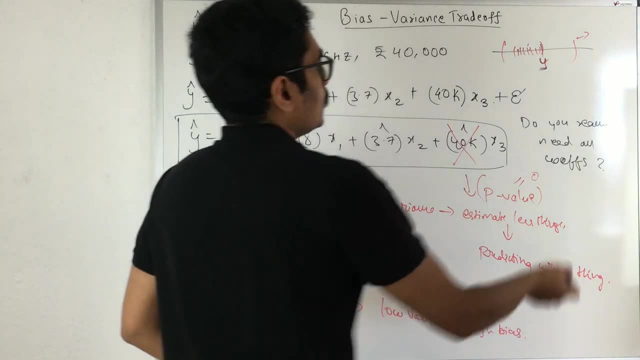 that you are not picking up the best one, but it may end up like you picked up some model from in between, but it may not be satisfying all the requirements that you want to have. So obviously, the second range, which is a very wider range, 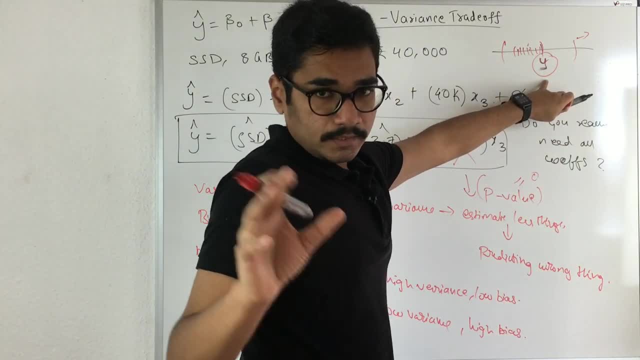 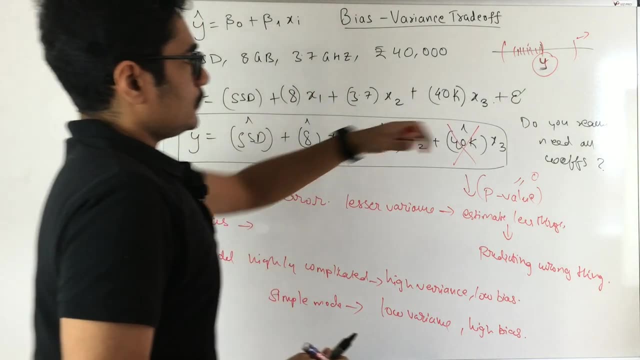 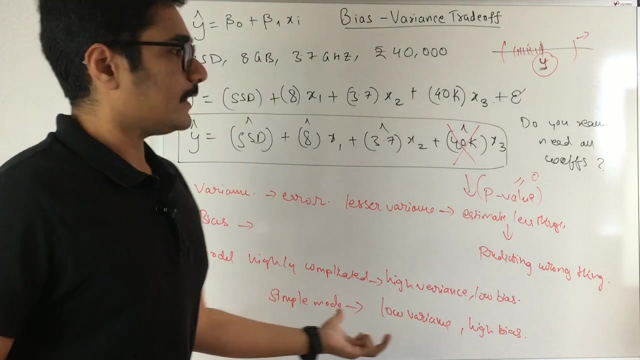 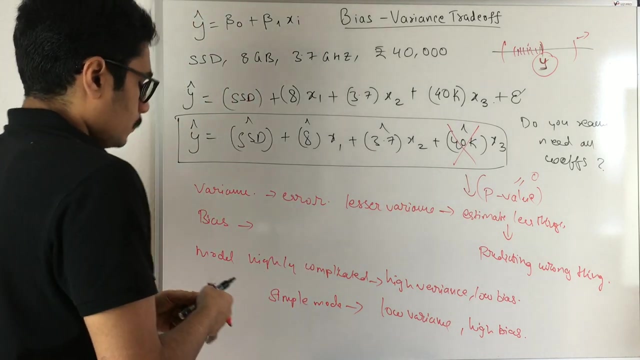 It also includes the actual thing or actual configuration which you want. So you will go with the second one. So this is the idea of what the bias and variance actually is. So this is how the entire idea is and say: if you want to implement this thing in calculations,